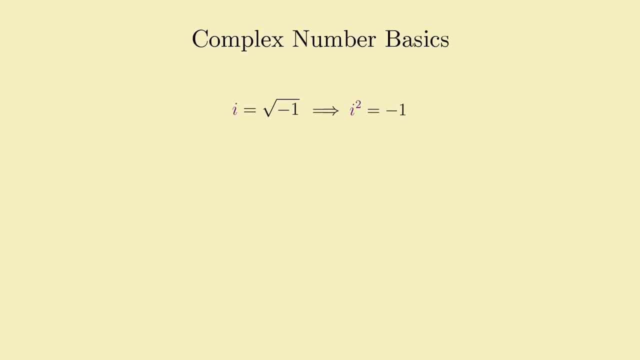 property that multiplying it by itself yields negative 1. It can be added to itself and multiplied by real numbers to get other imaginary numbers that are multiples of i, like 2i, 3i, negative 4i or 6.28i, You get a so-called 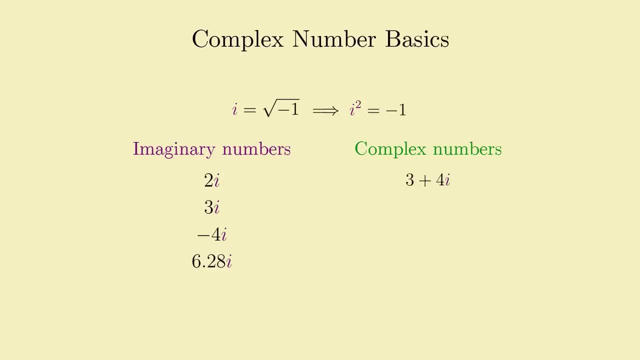 complex number by adding a real number and an imaginary number together, like 3 plus 4i or negative 1 plus 1.5i. These expressions are treated as atoms. They don't simplify any further and you can visualize them as points in the 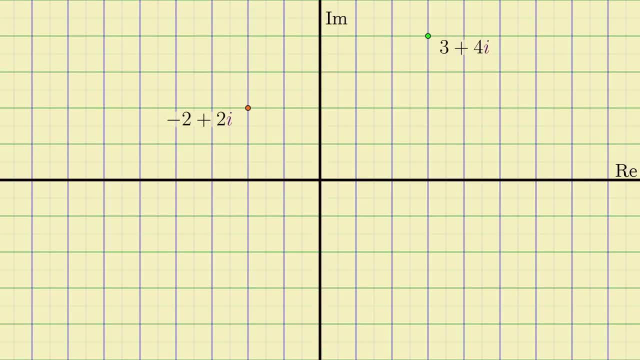 complex plane where the x-axis tracks the real part and the y-axis tracks the imaginary part. From this perspective, we can define the absolute value of a complex number as how far away it is from zero or the origin within this grid system, which you can compute by using the Pythagorean theorem on both the real 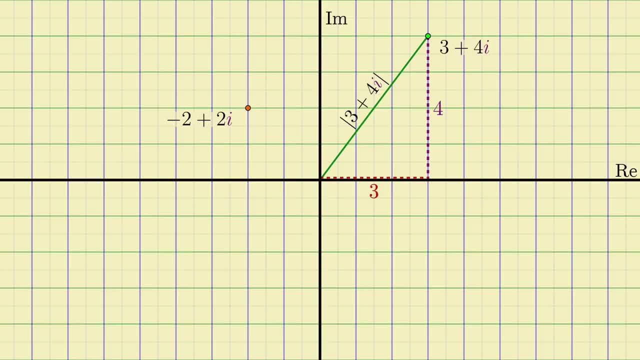 and imaginary parts. So, for example, the absolute value of 3 plus 4i works out to be 5.. Now two complex numbers can be added together by adding their corresponding real and imaginary parts, similar to how adding two vectors works. But unlike vectors, you can also multiply complex numbers together to get. 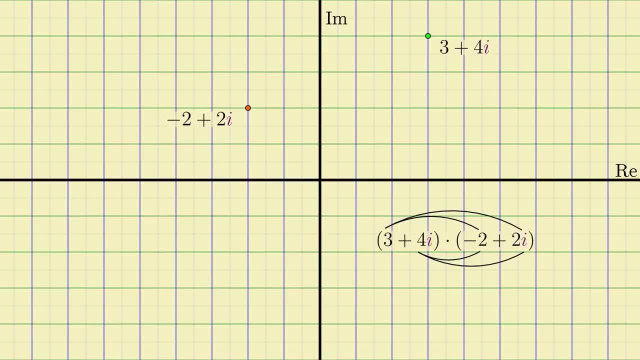 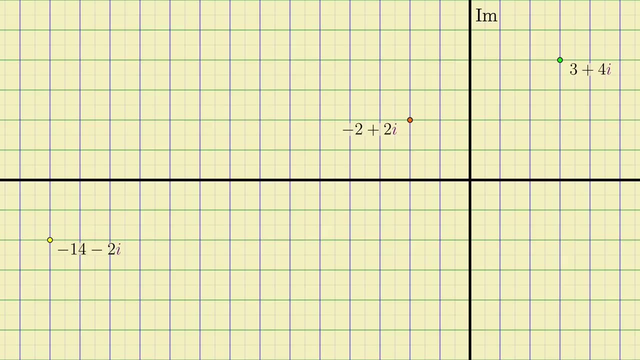 another complex number, and it works how you might expect, by following the distributive rule and remembering that i squared is actually negative 1, and simplifying from there. It might not be clear yet what complex number multiplication means geometrically just looking at these three points, but it actually has a very straightforward. 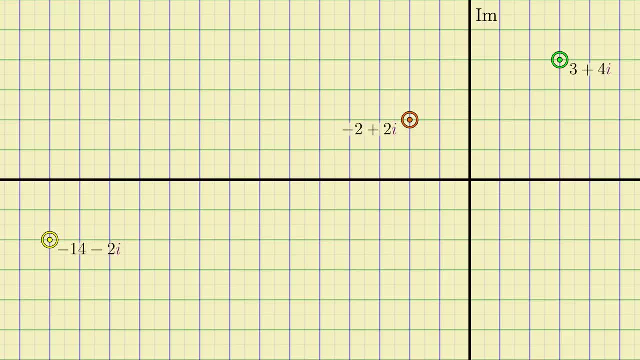 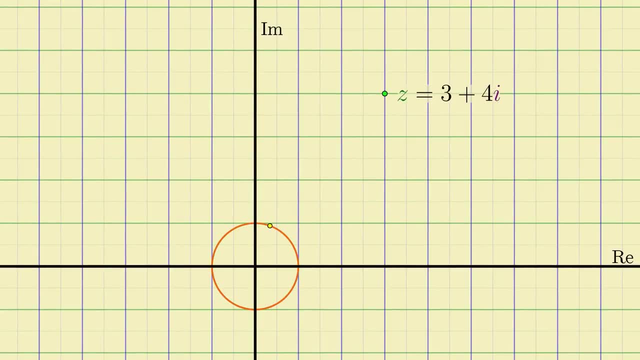 interpretation, which will be key to their geometric usefulness. To understand it, take a complex number- z, like 3 plus 4i here, and multiply it by a complex number w that sits on the unit circle. That is a complex number whose absolute value 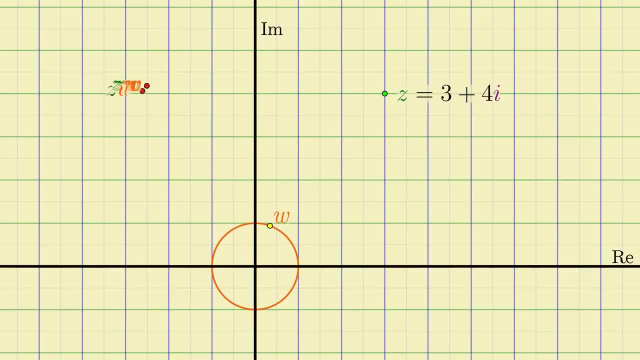 is 1.. You might notice that the product zw looks like a rotated version of z And indeed it is In fact. multiplying z by w, rotates it around the origin by the angle w makes with the positive real axis, in this case an angle of 70 degrees. So multiplying a complex number. 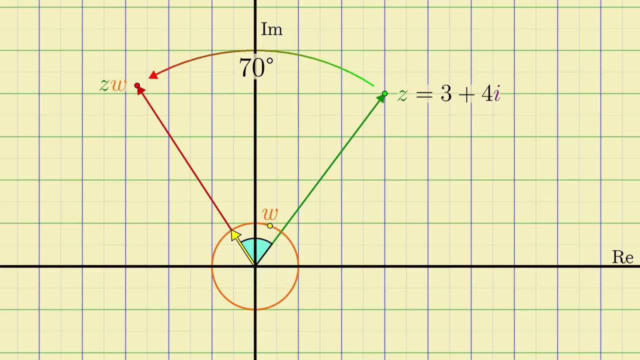 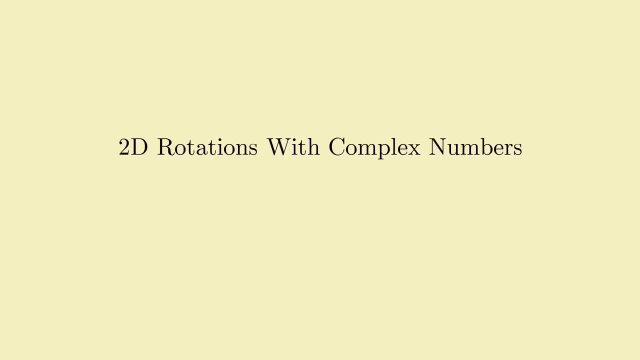 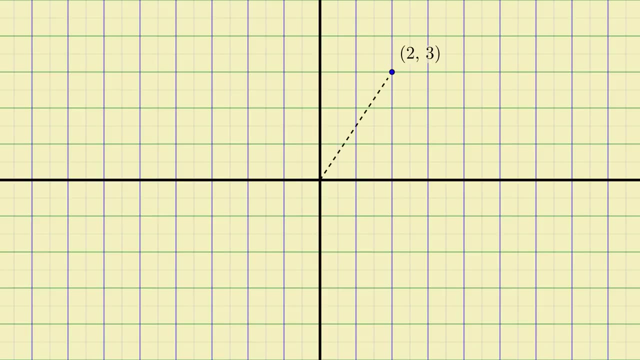 by a complex number of absolute value, 1 just rotates it. This makes complex numbers a useful tool for representing and computing two-dimensional rotations. For example, if you want to calculate the coordinates of where a point like 2,3 ends up after being rotated, say, 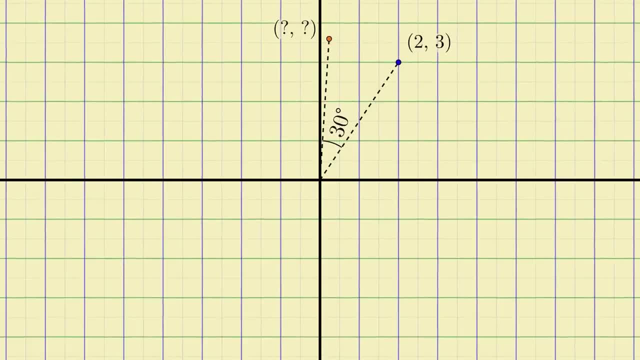 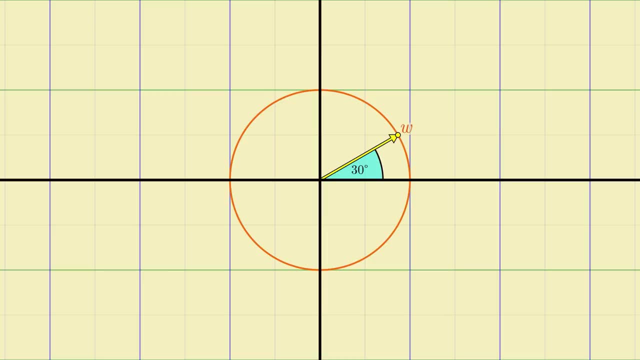 30 degrees counterclockwise around the origin. all you need to do is find the complex number on the unit circle, that is, 30 degrees counterclockwise off the positive real axis, and multiply it by 2 plus 3i. If you know a little trigonometry, this isn't too hard to do. 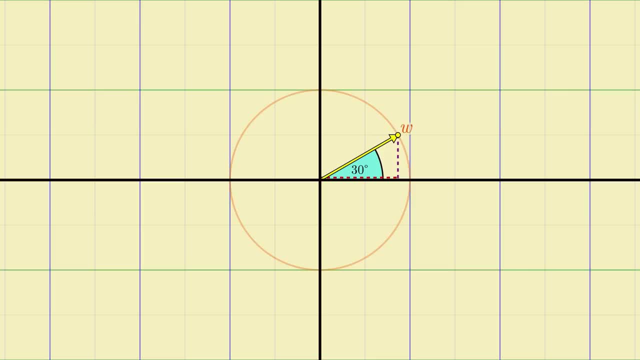 The xy coordinates of the point, 30 degrees along the unit circle are given by the cosine and sine, respectively, of 30 degrees, which work out to be about 0.87 and 0.5.. So our point w can be expressed as the complex number 0.87 plus 0.5i. 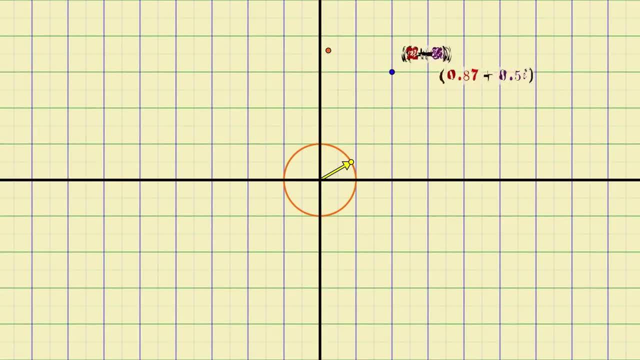 Multiplying it by our original point 2,3, expressed as the complex number 2 plus 3i, we get that it's about 0.2 plus 3.6i And looking at the picture, it matches up with where 2,3 ends up after. 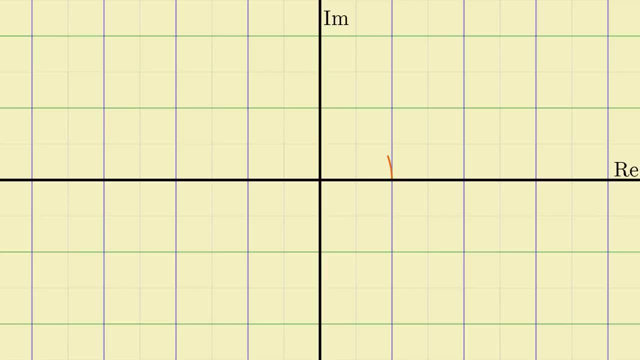 being rotated 30 degrees. Now, since this is such a common thing to do with complex numbers, it would be handy to have a shorthand way to refer to the complex number on the unit circle that is a given angle: theta away from the real axis. 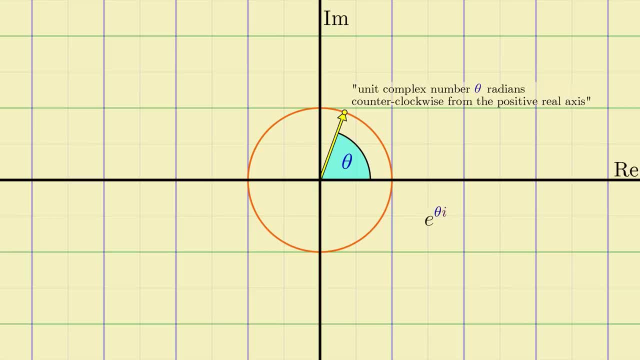 And luckily we have one. If you raise e to the power of the imaginary number theta i, where theta is measured in radians, the complex number you get is cosine of theta plus i sine of theta, which are the precise coordinates of the point we want. 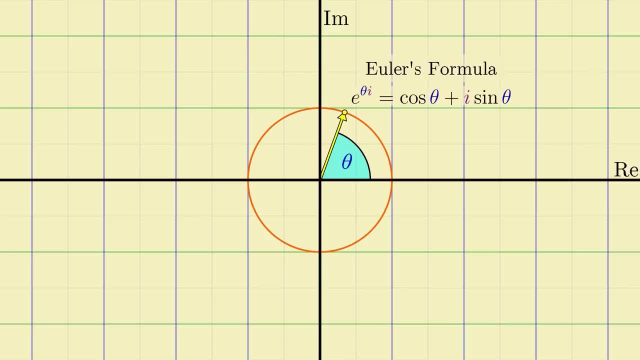 This relationship is called Euler's formula. Now I won't go into why Euler's formula is true in this video. Anyway, there are already many other resources that can explain it, probably better than me. But for now you can think of e to the theta i as a funky way to represent the complex number on the unit circle. 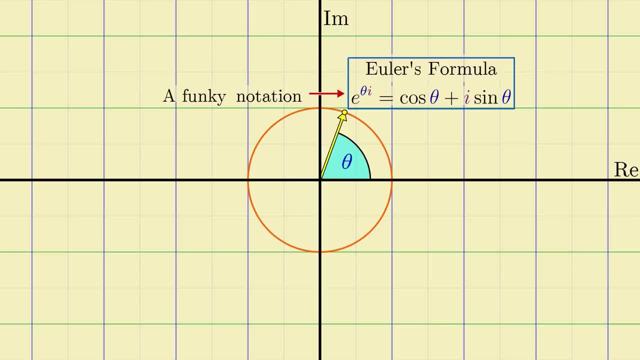 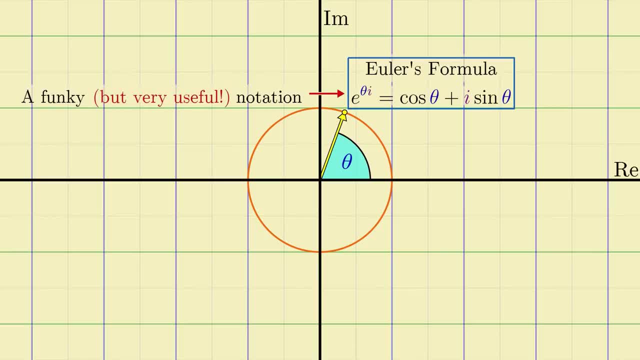 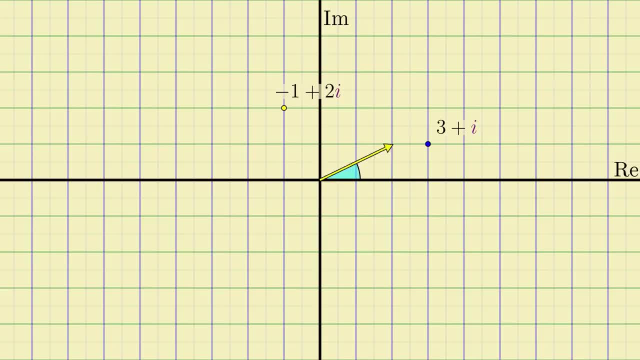 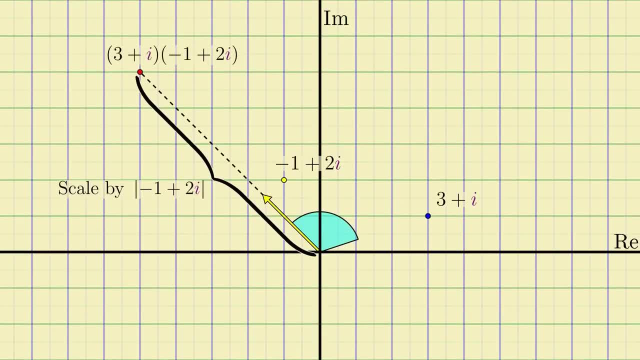 E to the theta i, E to the theta i, E to the theta i, by the absolute value of the number that multiplied it. For example, multiplying the complex number 3 plus i by negative one plus two i produces negative five plus five i, which is what you get by rotating three plus i by the angle. 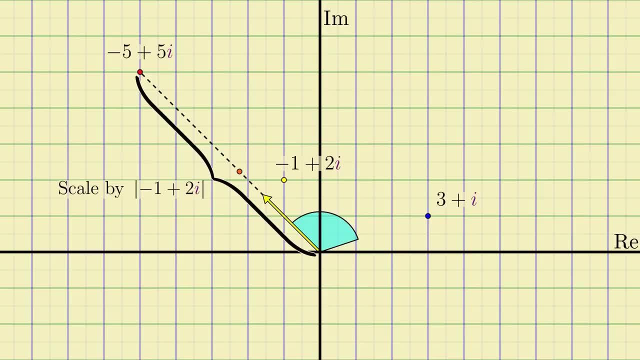 negative one plus two, i makes with the positive real axis and then scaling it up by the absolute value of negative one plus two, i, which is square root of five in this case. This is the key geometric interpretation of complex number multiplication. Multiplying by a complex number rotates and scales a point as opposed to real number. 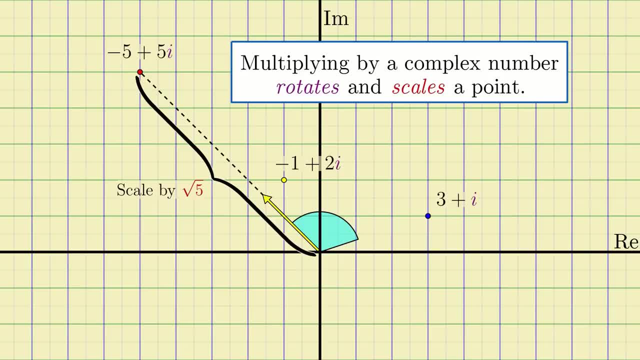 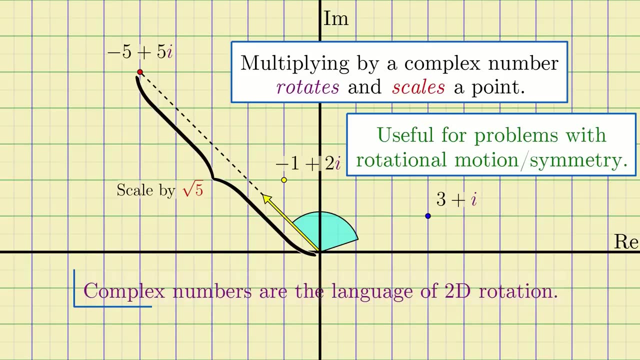 multiplication, which only scales. So complex multiplication provides a very natural way to describe two-dimensional rotations and because of this complex numbers are often super useful for problems involving rotational motion or rotational symmetry. Complex numbers are the language of 2D rotation. Subtitles by the Amaraorg community. 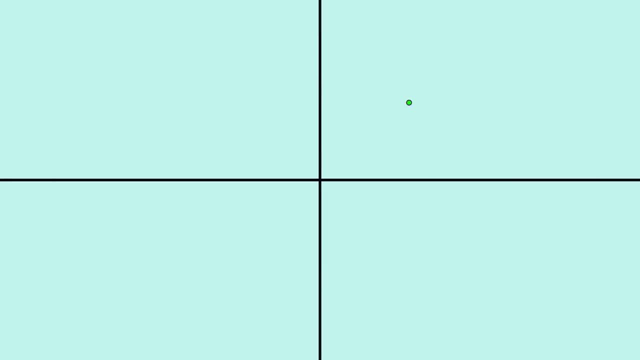 To see what I mean. consider this example. Let's say you have a point moving in 2D space around the origin in some kind of irregular way. Maybe it represents the motion of a charged particle in an electric field or something, Let's say the point's xy position. at any time t is given by two functions, x and y. 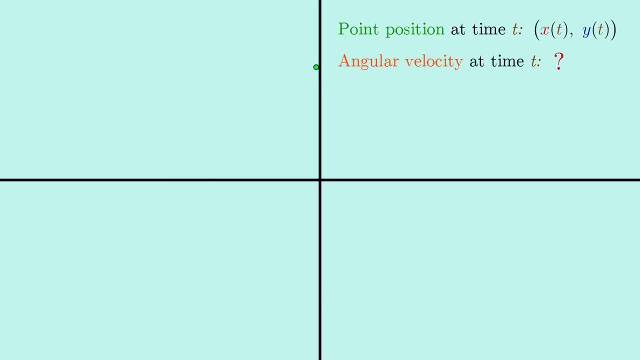 and we want to compute its angular velocity around the origin at any time. t, That is how fast the angle it makes with the positive x, is The x-axis is changing at any given moment or the time derivative of the point's angle function. 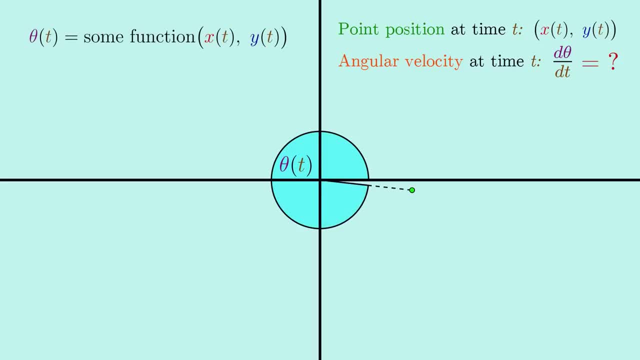 To compute this, we would presumably need to first calculate the point's angle function at any time t from its two xy position functions, so we can then take its derivative. There is some subtlety required to do this right, which I'll skip over, but it can. 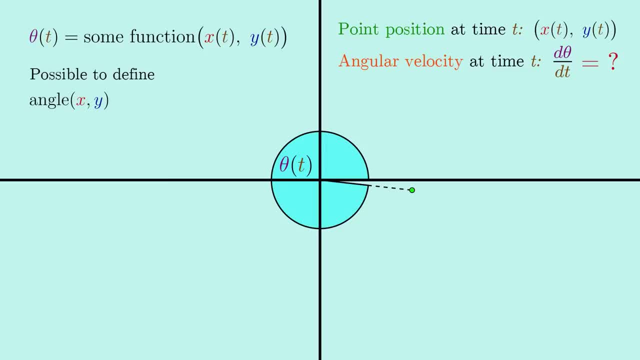 be done? It's possible to define a function that takes the xy coordinates of a point and outputs an angle in the range of x and y. The xy coordinates of a point are 0 to 360 degrees or two pi radians representing the counterclockwise angle. the point makes with the positive x-axis. 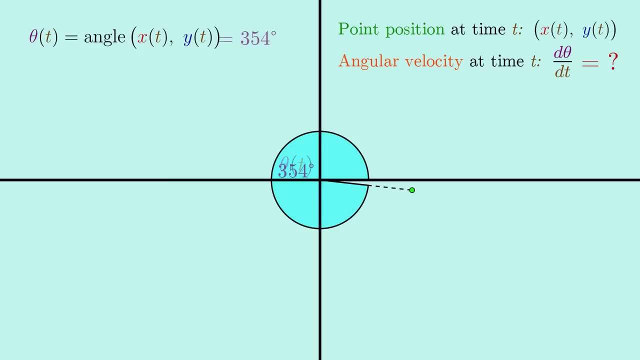 Throw in x and y into this function and we have our angle function, theta. But here we run into a subtle problem. This angle function is not continuous. If x is positive and y moves from being negative to being positive, then the angle function 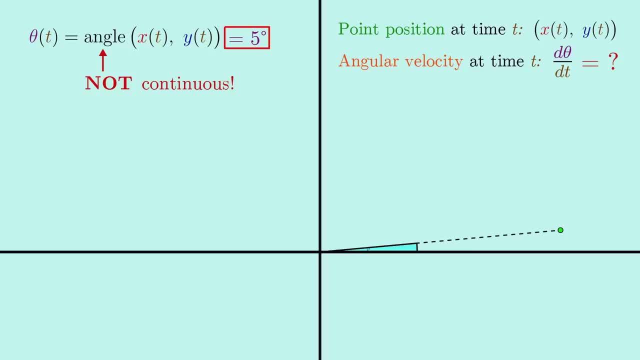 is positive, The computed angle will abruptly switch from being around 360 degrees to being around zero degrees. So if you're trying to measure the angular velocity by, say, measuring how much the angle changes in a short period of time, but the point happens to be very close to the positive- 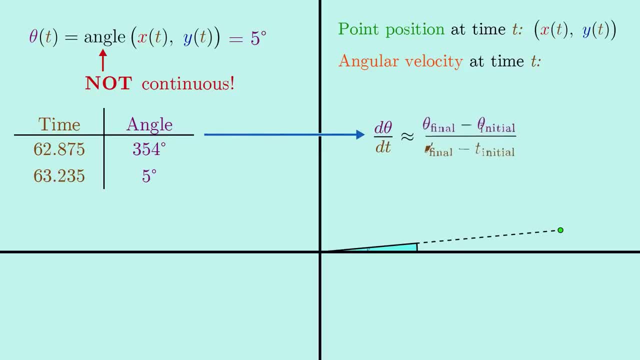 x-axis, you can wind up comparing angles from two sides of the seam and accidentally calculate a wildly wrong angle difference. What we'd really like is for the angle function to NOT be positive, So we can just take the angle function and put it in the positive x-axis. 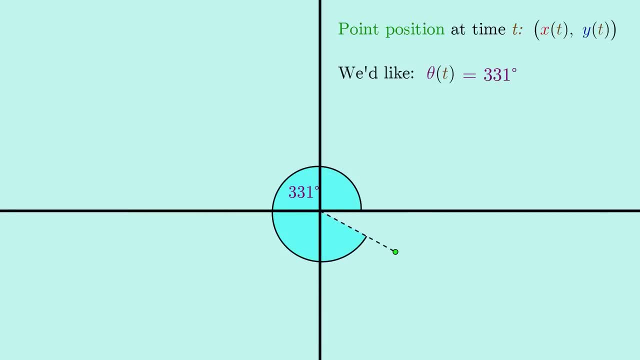 That's it. We can't wrap around to zero if we started from around 360 degrees, But unfortunately there's no way to easily do this. Angles are cyclic by their very nature. 405 degrees is the same as 45 degrees, and there's no real way to tell the difference. 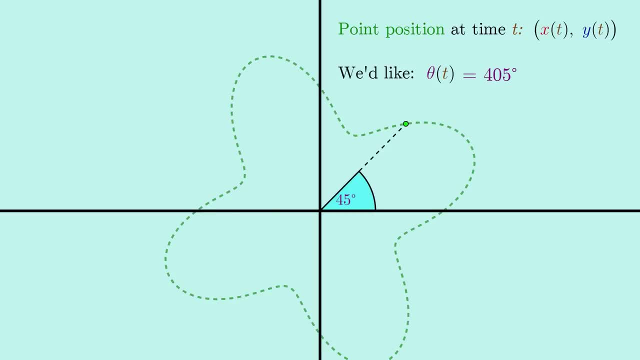 between them, without remembering the entire prior history of the point's motion, which would be a hassle. So are we stuck then? Is there no easy way to calculate a local change in angle? Is there no way to calculate a local change in angle? 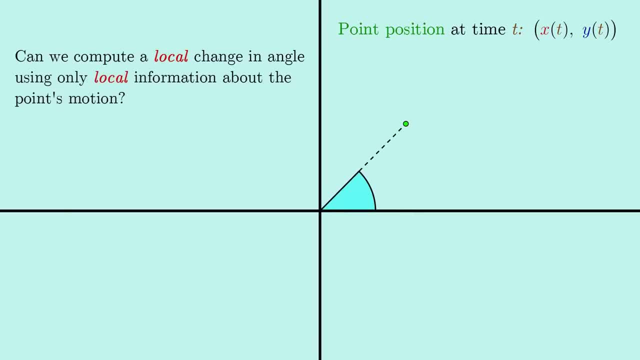 Is there any local information about the point's motion? Well turns out there is a way. The trick is to calculate the derivative of the angle function indirectly, without knowing its full angle function in advance, And complex numbers provide a sneaky way to do just that. 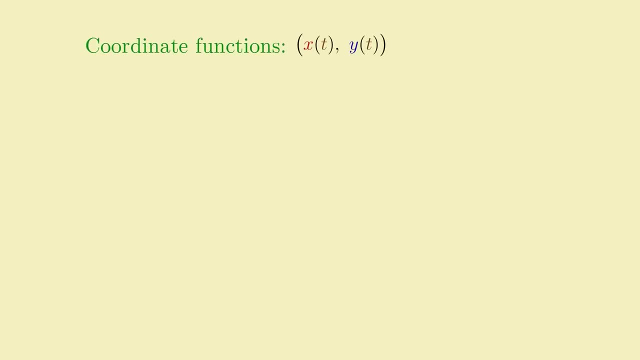 To do it, first package our two coordinate functions x and y into a single complex-valued function, f, which outputs x plus i, y for any given t-value. Now observe that we can always express a complex valued function in polar form as r of t times e to the i theta of t, where r of t is just. 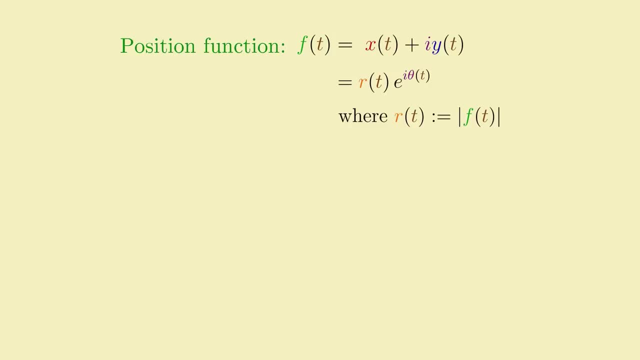 the absolute value of f of t, which is just square root of x of t squared, plus y of t squared in this case, and theta of t is the full angle function of the point which, remember, we're trying to avoid computing directly. If you take a, 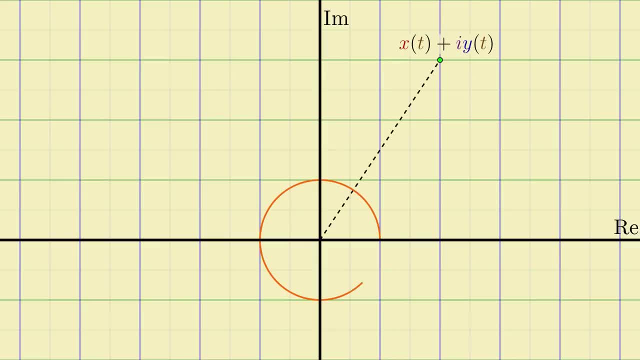 step back. this formula should make sense right e to the i. theta of t is a complex number on the unit circle that makes the same angle with the positive x axis as our point and if we scale it up by r of t, the point's distance from the. 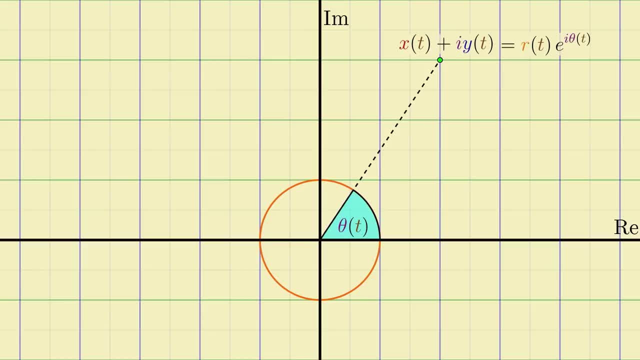 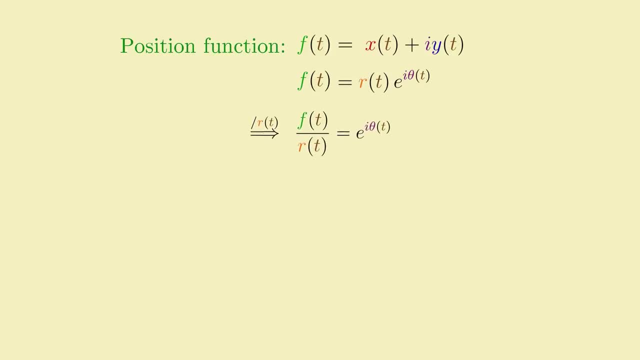 origin, it will coincide perfectly with our point. Okay, now here comes the trick. Take this polar equation for f of t and divide both sides by r of t to get f of t over r of t equal to e, to the i theta of t squared squared plus y of t squared squared. 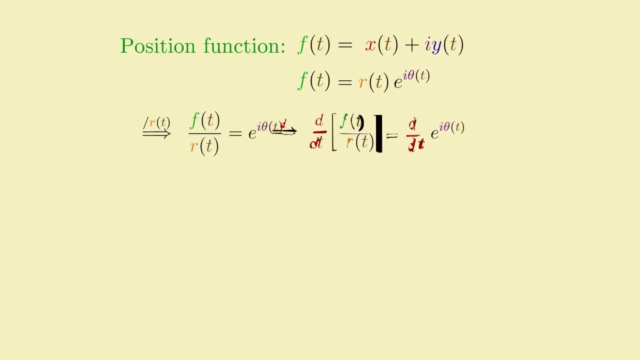 Now we'll take the derivative of both sides. One of the really nice things about complex numbers is that many of the algebra and calculus rules you're used to for real numbers and functions work in exactly the same way in the complex setting, and derivatives are no exception, Even though 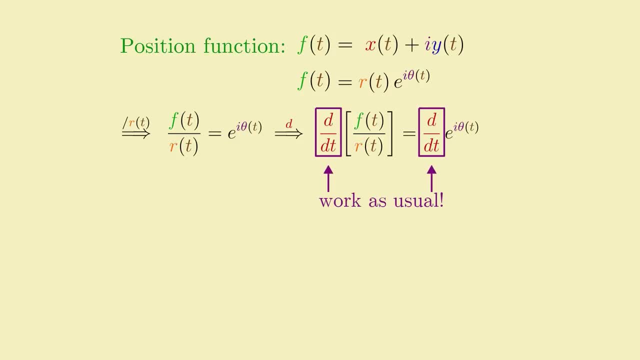 all the functions here are complex valued, the familiar derivative quotient rule applies. so on the left-hand side we get the usual expression: f prime, r minus f of t squared, squared, squared, plus y of t squared, squared, squared. But what's really cool is the exponential derivative rule works the same old way as 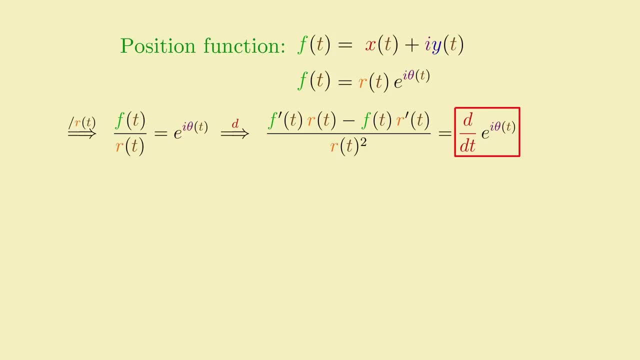 well, On the right-hand side, the derivative of e to the i theta of t will just be itself times the derivative of i theta of t, in accordance with the chain rule. And since i is a constant, it just becomes i times the derivative of theta. Do you see now why writing a unit-complex? 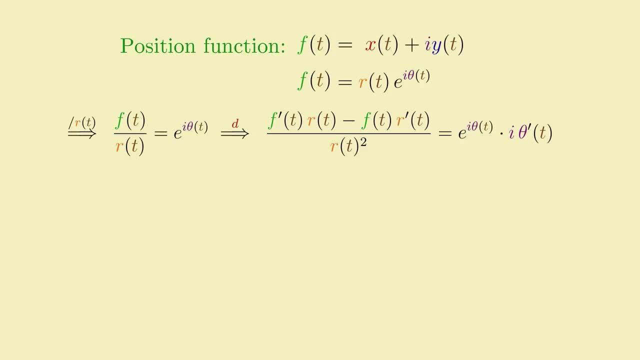 number as e to the i theta is so easy. Now remember: our goal is to compute theta, prime of t, the derivative of theta, without having to know what theta of t is in advance. And at this point we can actually get rid. 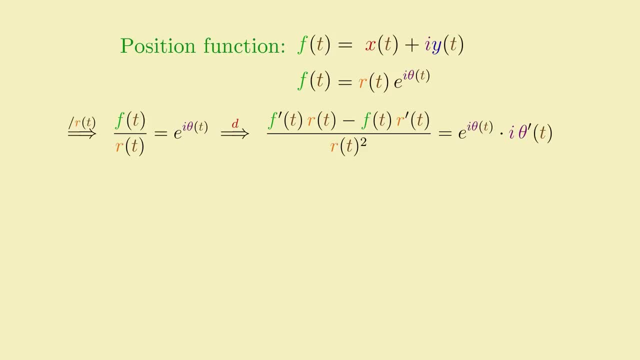 of the explicit theta of t that remains in the equation. Before we took a derivative, remember how we had f of t over r of t, equal to e to the i theta of t. Well, it means we can substitute f over r for e to the i theta of t. 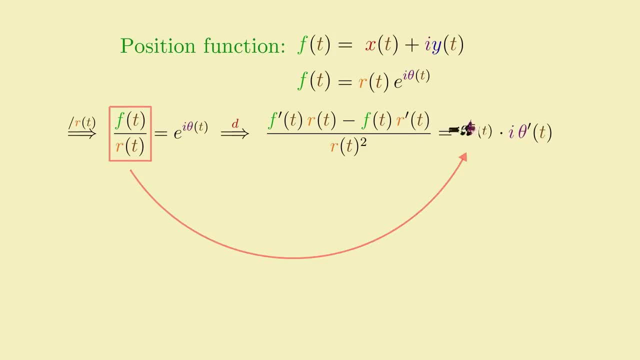 So we can compute theta prime of t over r of t times f of t over r of t times theta prime of t equal to the quotient mess on the left-hand side. From here, with a little rearranging you can solve for i theta prime of t and get. 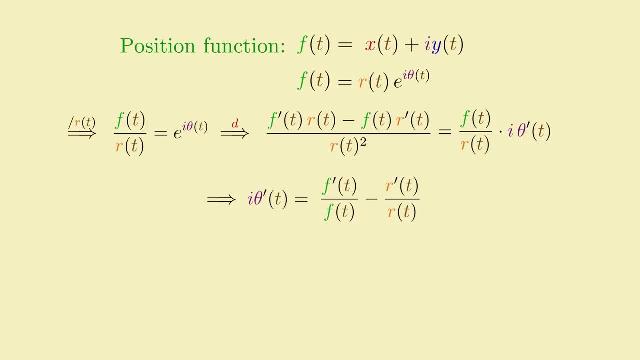 that it equals f prime over f minus r prime over r. But now we can make an interesting observation: Although f and f' are complex-valued functions, theta prime of t are purely real-valued By themselves, r and theta prime just. 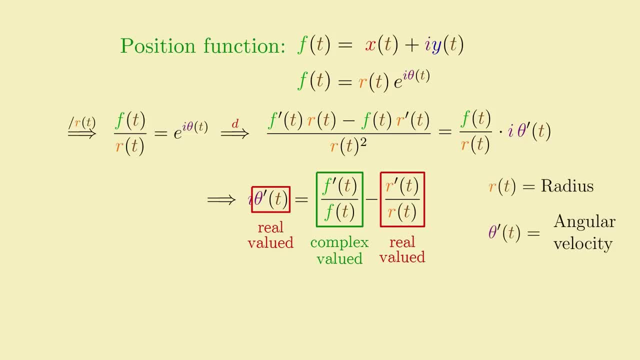 represent radius and angular velocity of our moving point. Perfectly real, nothing complex about them. And since our real-valued theta prime of t is being multiplied by i on the left-hand side, the whole expression must be purely imaginary. so theta prime itself can be extracted by taking the imaginary part. 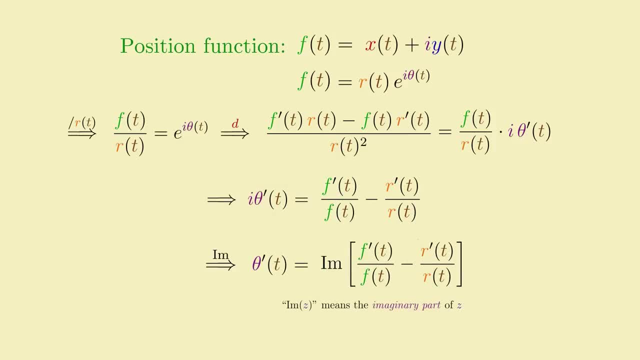 of both sides, And since r and r prime are both purely real-valued functions, subtracting r prime over r will have no effect on the imaginary part of f prime over f, so we can just drop it And in the end we get a really nice, compact little. 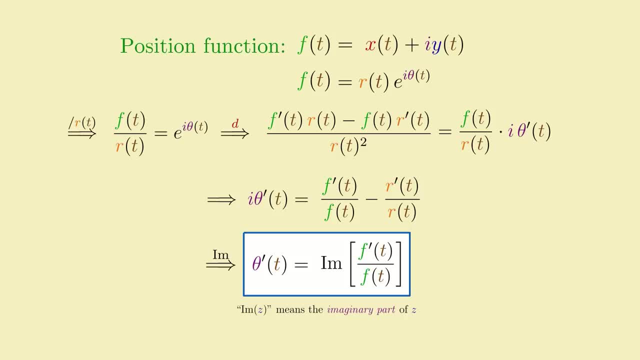 formula that will compute the derivative of theta directly from f, prime and f without having to touch the original full theta function at all. And remember f of theta is the derivative of theta and f of theta is the derivative of theta. And remember f of theta is the derivative of theta and f of theta is the derivative of theta. 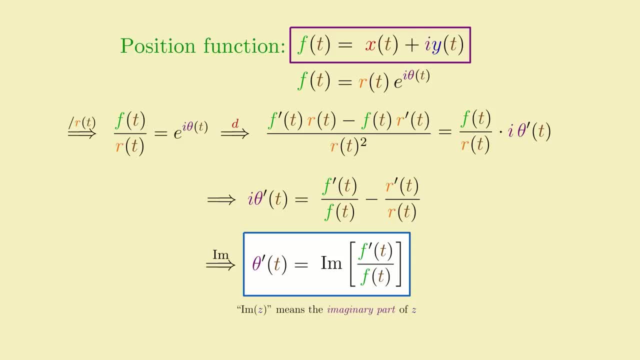 f of t is really just x of t plus i, y of t, So really, we've found a way to compute the angular velocity directly from the x and y coordinate functions. Isn't that neat. But does this formula really make sense, though? I mean, if we 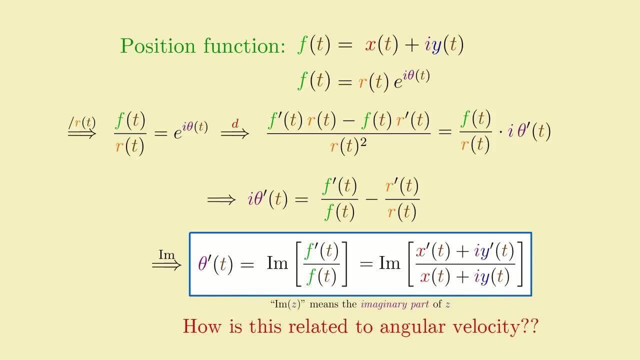 take a step back. why should this wacky expression have anything to do with angular velocity? And if you don't know calculus, this may all seem like black magic anyway. So let's see if we can figure out what each piece of this formula. 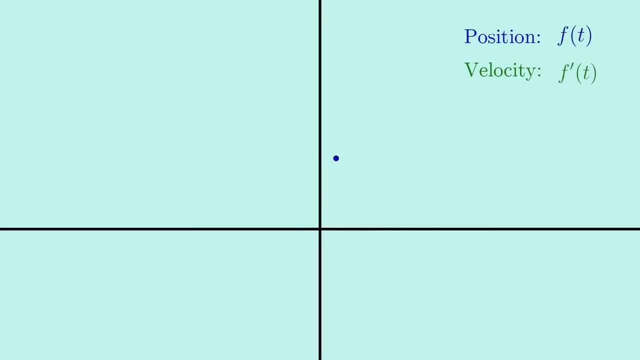 is doing and why. f of t and f prime of t represent the position and velocity of the point at any time, t. So let's label them in the picture with two vector arrows: blue for position, green for velocity. Now in our formula for angular velocity we divide f prime of t, the velocity. 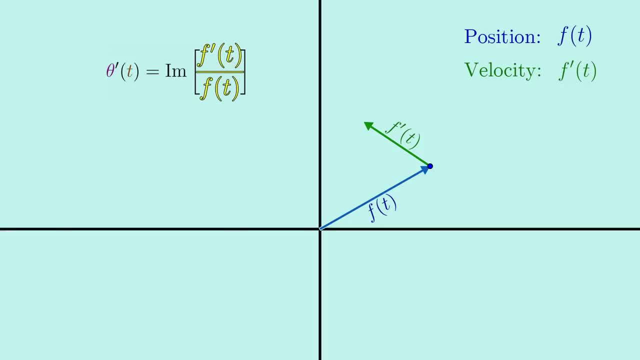 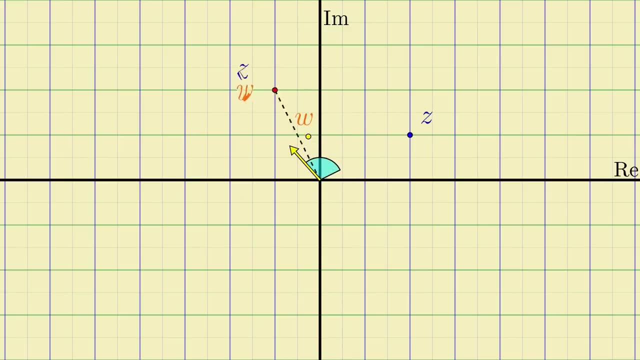 vector by f of t, the position vector, Ignoring scaling. remember that multiplying by a complex number results in a rotation, A rotation by the angle it makes with the positive x-axis. So dividing by a complex number does the opposite: A rotation by the same angle, but in the opposite direction. 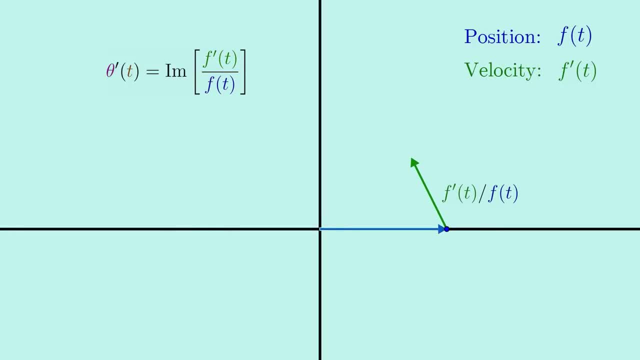 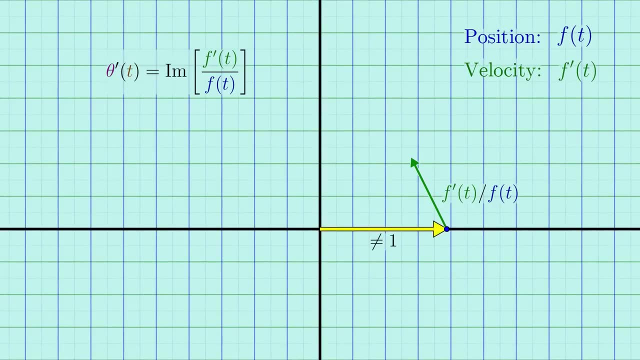 So dividing f prime by f rotates the velocity vector backward by the position vector's angle. Now, since the position vector is presumably not a unit vector, dividing by it will also scale the velocity vector down by the magnitude of the position vector. But let's ignore that for the moment. 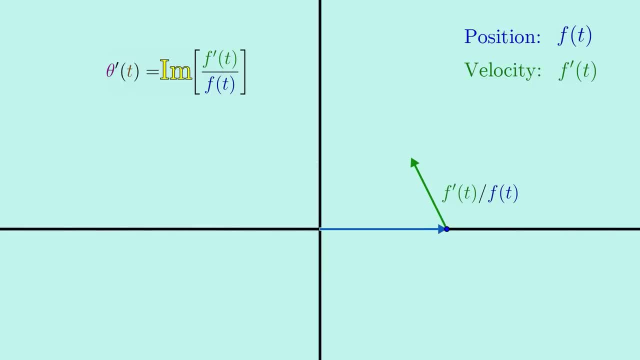 Continuing with our formula, we then take the imaginary part, which grabs the vertical component of this rotated velocity vector. But since the velocity vector was rotated backward by the angle of the position vector, the vertical component here really represents the component of the original velocity vector in the direction perpendicular to the position. 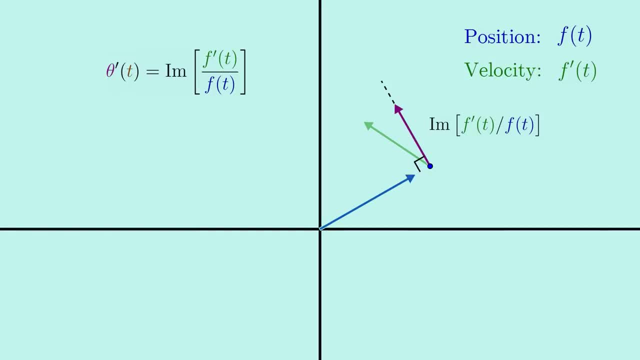 vector. And since the position vector always extends radially away from the origin, we can now see that the velocity component perpendicular to it really represents the circular component of the velocity vector around the origin at time t. But now remember that in reality, dividing by the position vector also scales the velocity. 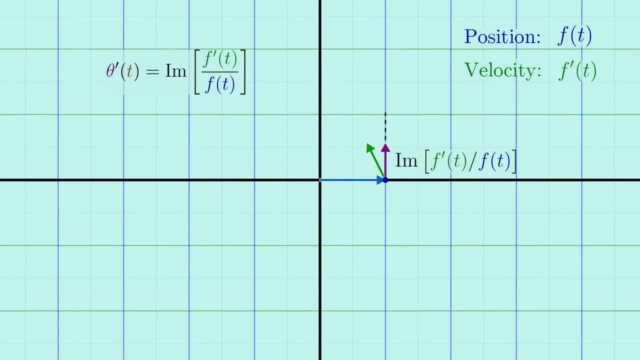 down by the magnitude of the position, that is, by the current radius of the point away from the origin. And dividing the circular speed of an object by its radius of rotation yields its angular speed, Just like how dividing the length of a circular arc by its radius yields the arc's angle. 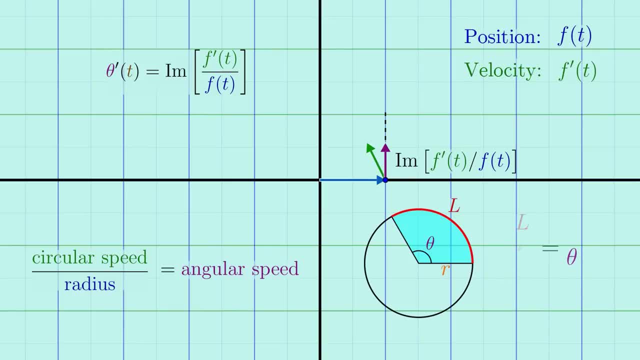 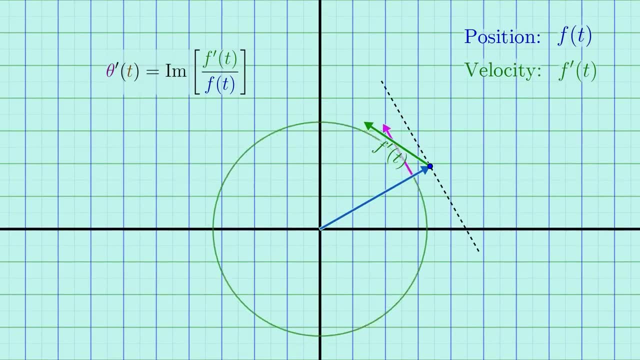 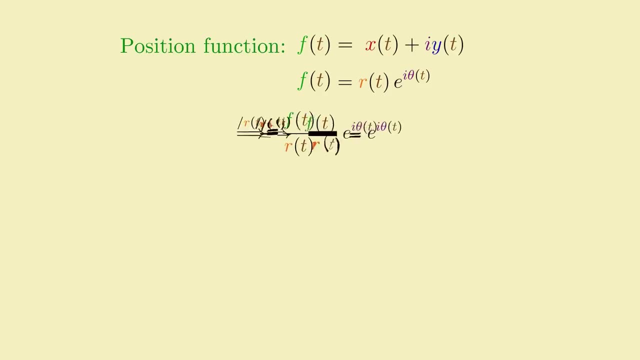 in radians. So this little formula is really a compact and elegant way to extract the circular component of velocity and then divide it by the radius to obtain an angular velocity. Isn't that clever? But what I love is how you don't even have to be that clever to come up with this formula. 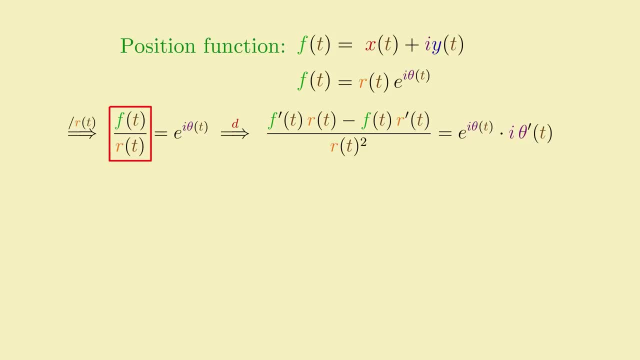 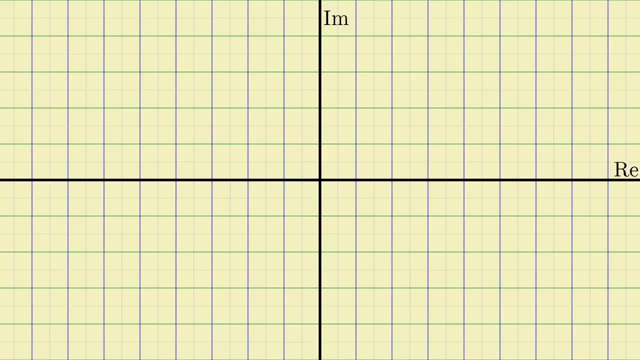 If you know calculus and aren't afraid to use complex numbers, this sneaky little formula will help you out. The sneaky little formula just pops out like magic from taking the derivative of the polar representation of the position function. If that's not a testament to the power of complex numbers, what is? 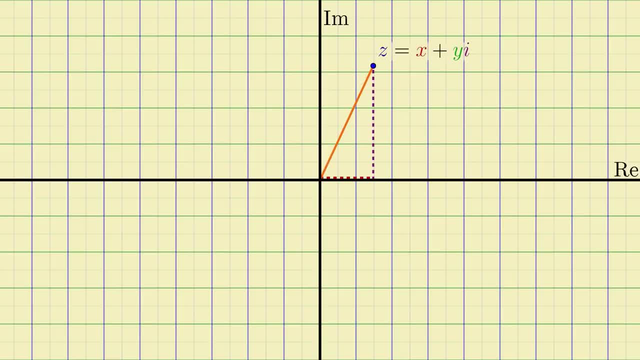 So I hope that gave you a taste for how complex numbers can succinctly describe geometric relationships and provide a really natural and elegant language to describe 2D rotational dynamics. But I could go on with so many other examples, Like how dividing two complex numbers can be a very simple task. 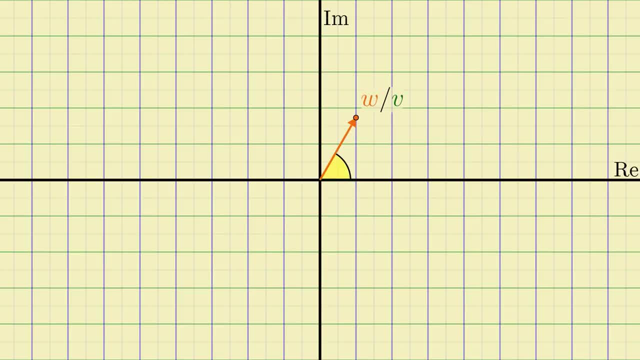 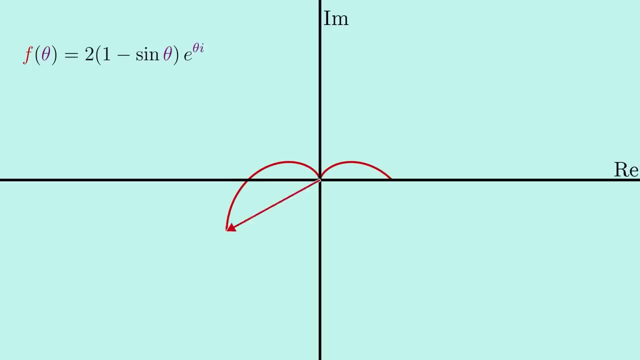 Or how dividing two complex numbers encodes the rotational action between them, providing a clean way to rotate a point by the angle between two vectors. Or how they provide a unified way to represent both rectangular and polar parametric functions, something we already saw a little in this video. 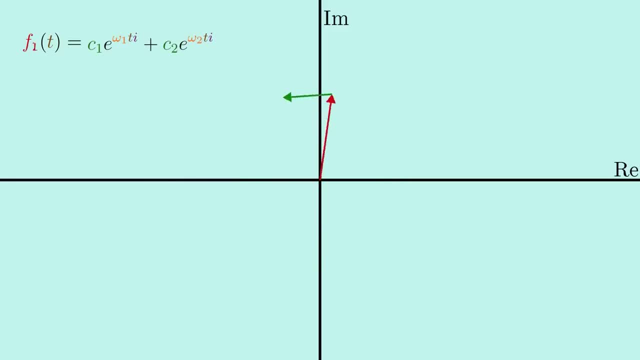 Or how they make describing epicycles really easy, which is essentially what Fourier series are built from: True, Truly Complex. It's a very simple language to describe so many two-dimensional scenarios, and I find them an indispensable tool for this reason. 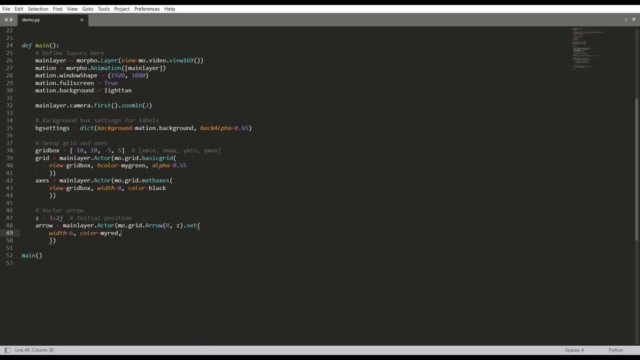 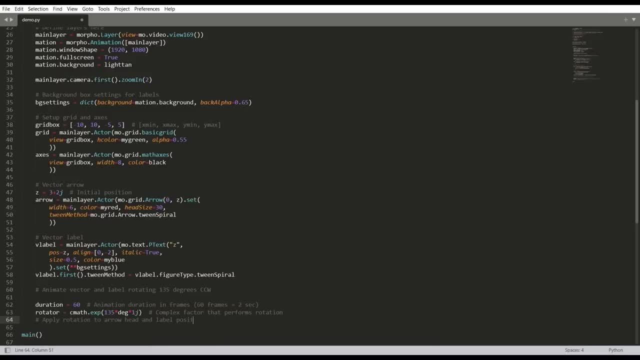 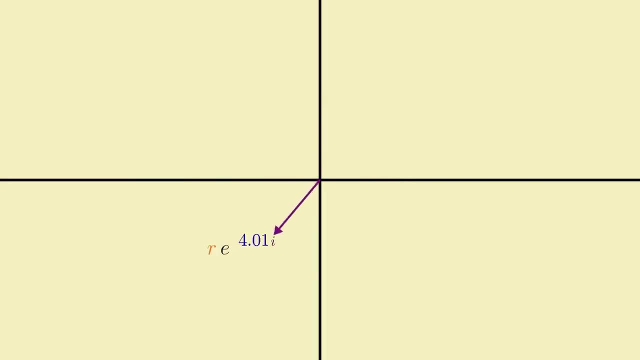 As a matter of fact, Morpho, the software library I wrote to create most of the animations in these videos, encodes almost all 2D positional data as complex numbers, just because it's so easy to manipulate in that form. But as great as complex numbers are, I should mention a limitation they have. 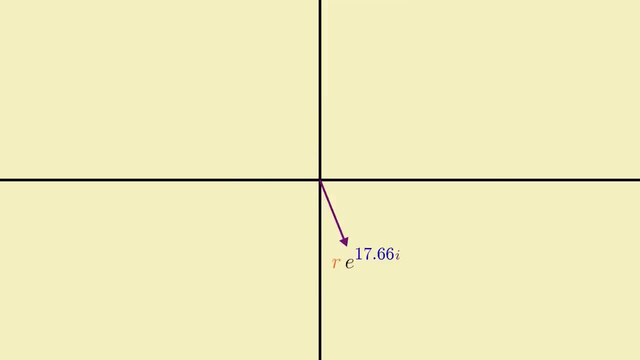 Although they describe 2D rotation extremely well, they're not as complex as they seem. They're not as complex as they seem. They're really pretty much limited to just 2D. By themselves, they can't faithfully describe 3D rotations. 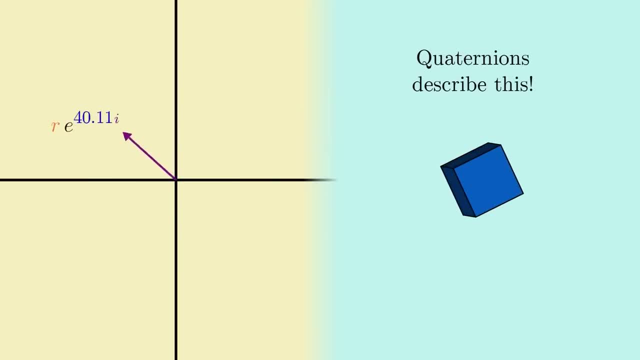 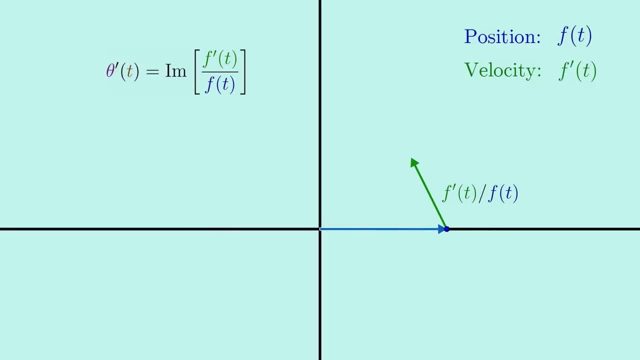 The tool for that is the quaternions, the big brother of complex numbers, which we don't have time to discuss in this video. Still, I hope you came away with a better understanding of just how wide the utility of complex numbers is and how much you could be missing out on without a working understanding. 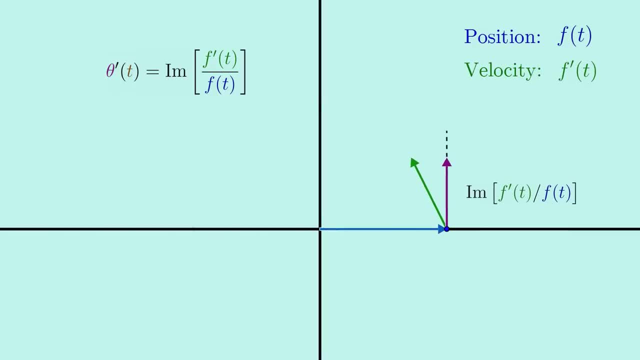 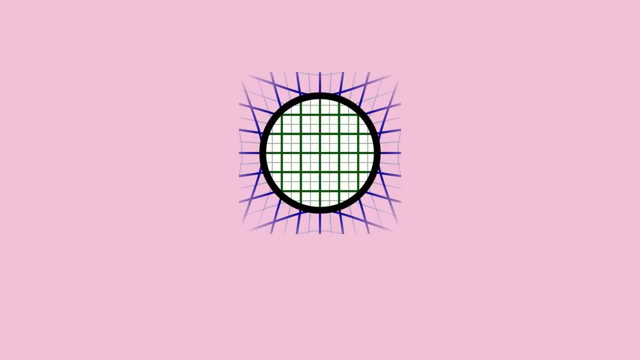 of them. Really, they don't have to be all that complex. And why not? Because once you get used to them, they start to feel like old friends. Hey everyone. So I have a bit of an announcement to make. Morphocular now has a Patreon page. 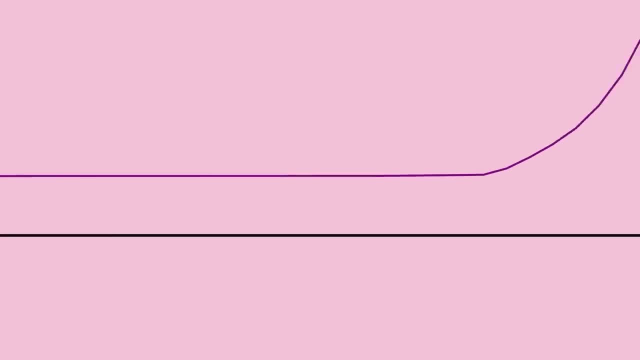 Over the past several months. it's pretty fair to say I've been blown away by the impact and reception these videos have gotten, as evidenced by the recent rapid growth of this channel. It's been quite the ride for me, who hadn't dared hope to make such a large impact in